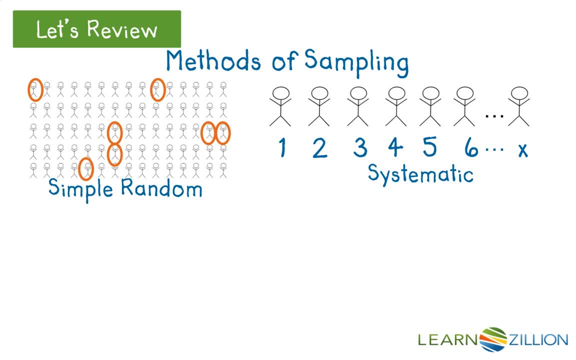 and we take every nth person and randomly choose where we put them. Here is how we begin. In this diagram we are choosing every third person Of the first three people. the second person is randomly selected as the starting point. So we would choose person number 2, person number 5,, person number 8, and so on. 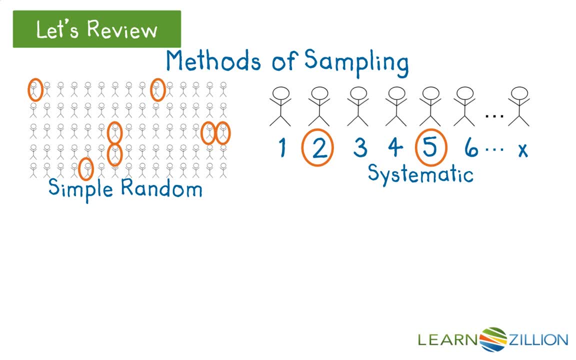 If we are choosing every 10th person, we must randomly select one of the first 10 people to start our sample. In stratified sampling we are using a simple random sample sampling. we divide our population into groups based on some characteristic. so 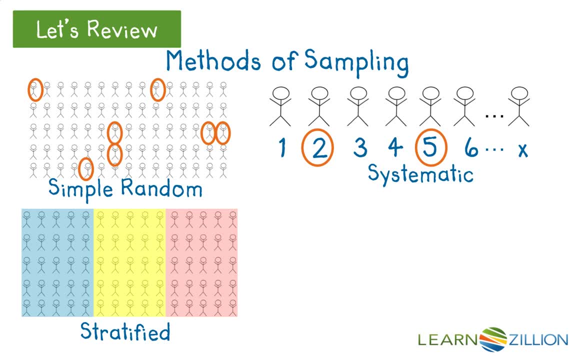 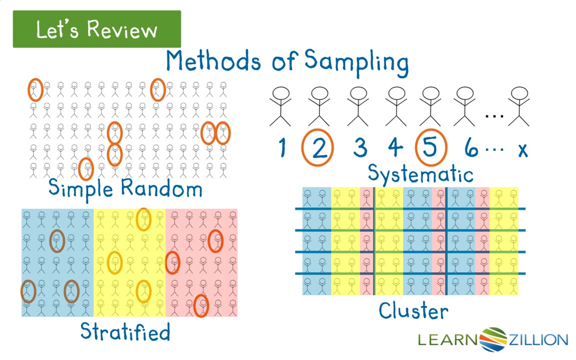 that the individuals in the groups are similar to one another and randomly select members from each group. in cluster sampling we divide our population into groups that are similar to the population in some way. often these groups are naturally divided, such as neighborhoods in a city or first period classes in a high school. then we randomly choose a specified number of. 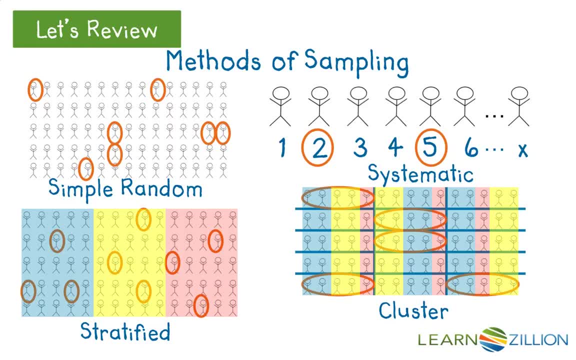 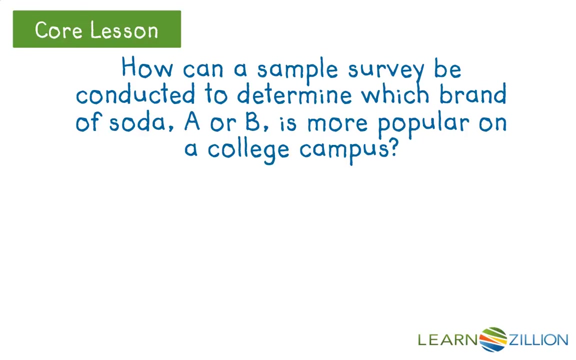 these groups or clusters to survey. there are also other methods of sampling, such as convenience and voluntary, but for the purposes of our problem these two have much more potential for bias, so we will not choose one of those for our sampling method. core lesson: how can a sample survey be conducted to determine which? 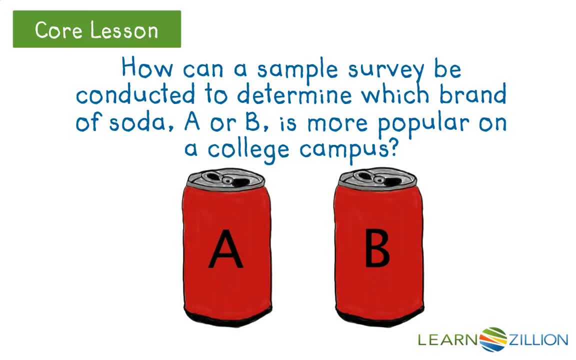 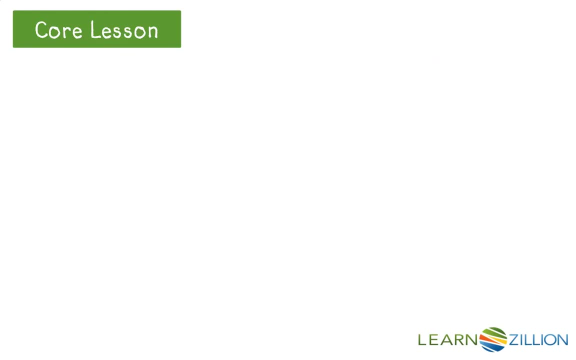 brand of soda A or B is more popular on a college campus? we want to find out which soda is more popular, so we will look for student opinions. the best way to find out someone's opinion is to ask them, so we will use the survey. first we must 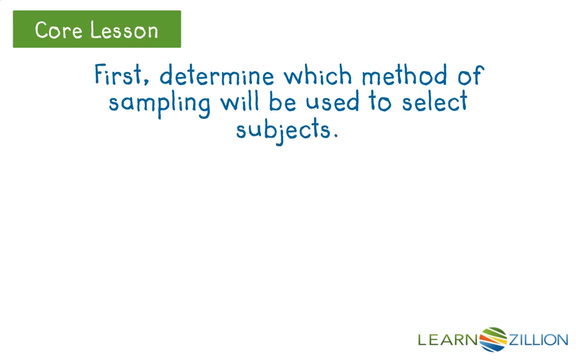 determine which method of sampling will be used to select our subjects, because we want to know which soda is more popular on a college campus. it may be difficult to conduct a simple, random sample of all the students if we put them into groups. there may be more potential for bias depending on how they are grouped. so we 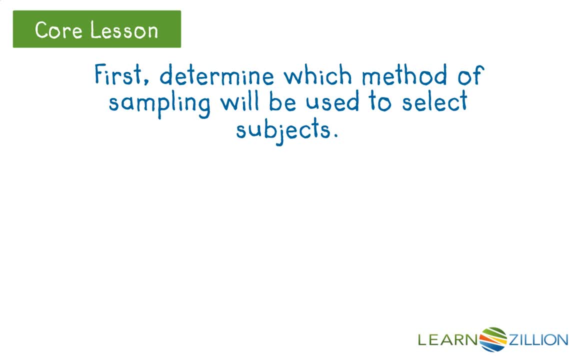 won't use stratified or cluster sampling for this problem. we will use systematic sampling. it just so happens that the student ID office is requiring each student to get a newly updated student ID, so all students will have the same opportunity of being selected. we choose to begin our study at 1102 am and we choose every fifth person who. 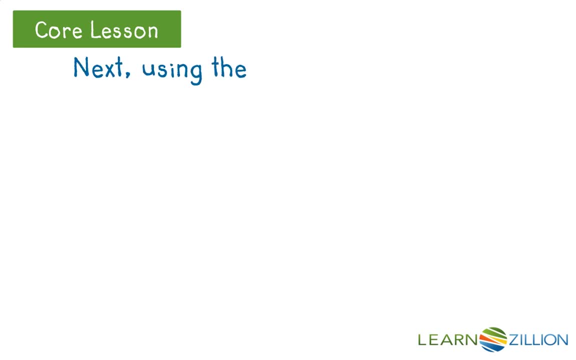 walks into the student ID office. next, using the selected method, we will ask the subjects which soda they prefer, A or B. when they enter the student ID office, we will give them a pen and one of two slips of paper which were randomly put into a stack and ask them to follow the directions. 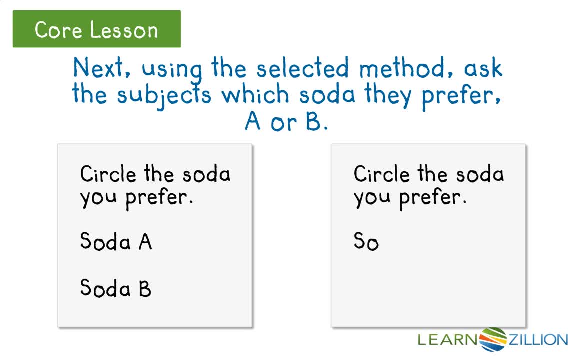 the two papers look exactly the same, only the order of the choices will vary, because they are reading the instructions and selections on the paper. this reduces any bias that may be inadvertently created by the surveyor asking the questions vocally. sometimes the inflection of our voice can cause. 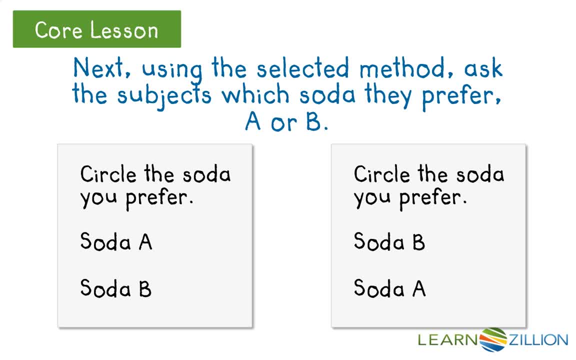 someone to choose differently than they originally may have. a common misunderstanding is to fail to randomly select our subject. this is an préfaried mistake of mine. I feel like I haven't been asked to grade it myself, so I didn't Validated by your test. YEAH. 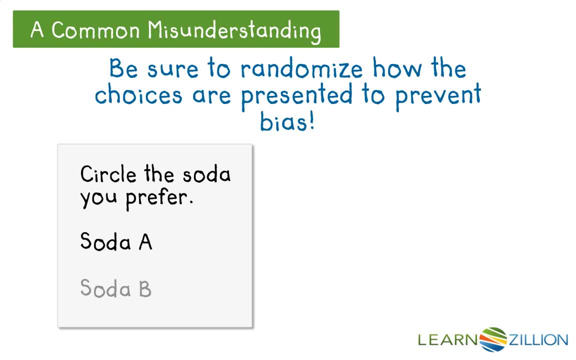 how the choices are presented. we randomly put the papers into a stack so the varied order of the choices would be distributed randomly. we want to avoid as much bias as possible. many people have a theory that on a multiple choice test, if you must guess, choose C because they think that answer is correct. on a higher 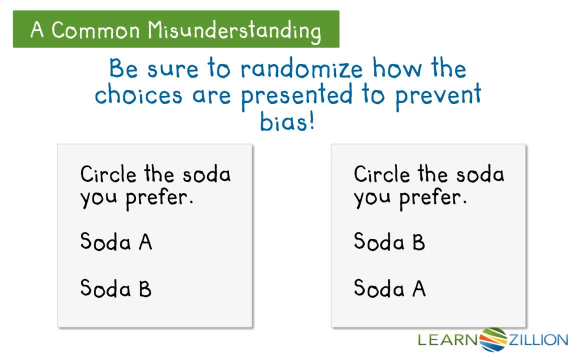 percentage of questions than any other choice. whether or not this is true is irrelevant. if many people believe it, they may choose C for solely that purpose. this is similar to why we want to randomize the order of our choices of sodas A and B. finally, draw your conclusion based on the data you've.